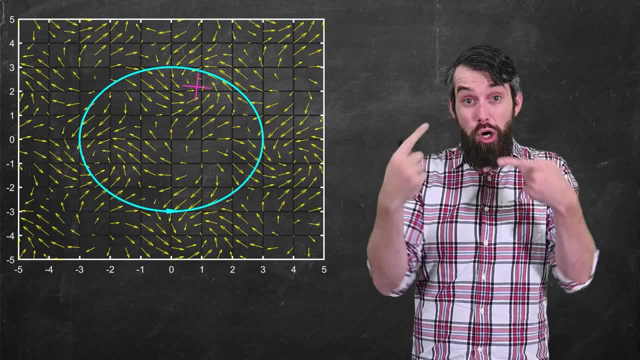 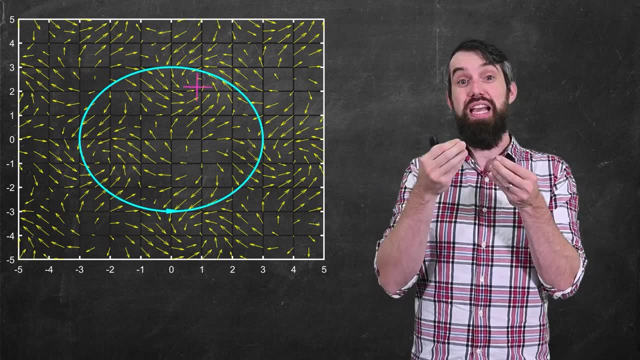 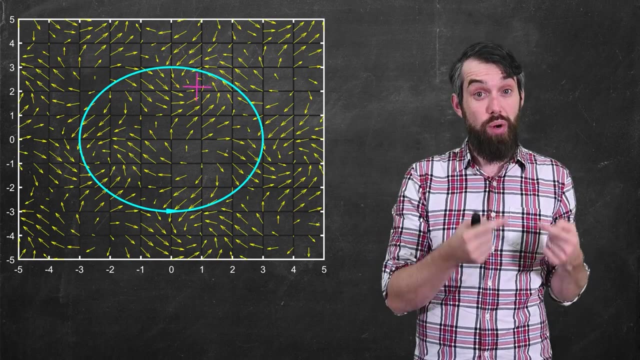 So here's the idea: Imagine I have a vector field and I have some curve that goes around the vector field. As I saw in the previous video where we introduced the notion of the circulation density or the curl at a particular point, we've seen that at any specific point I can measure the degree to which my field is causing a little propeller to spin at that particular point. 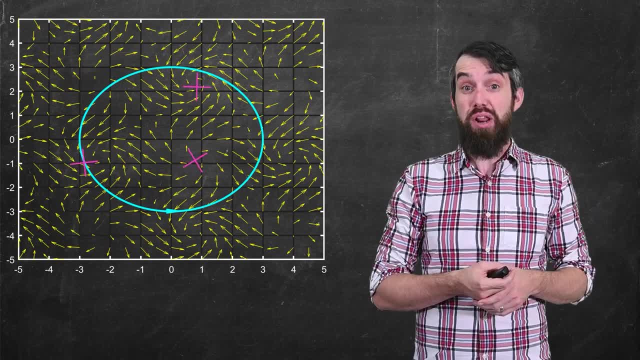 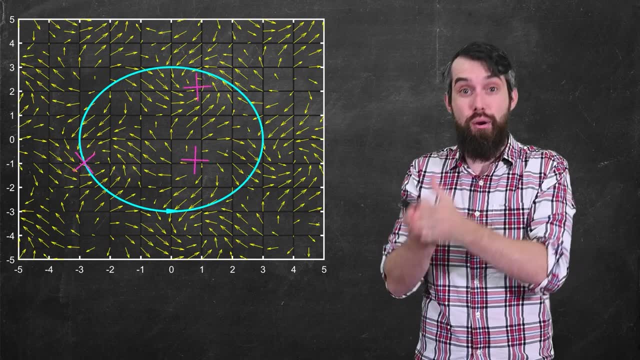 There's one spot and then we can look at a few others here and in fact we can put one right on the boundary if we so did. So, depending on what the field is, you go in and measure at some spot and put a little propeller there, it might rotate clockwise or counterclockwise, faster or slower, it just depends on what the underlying field is. 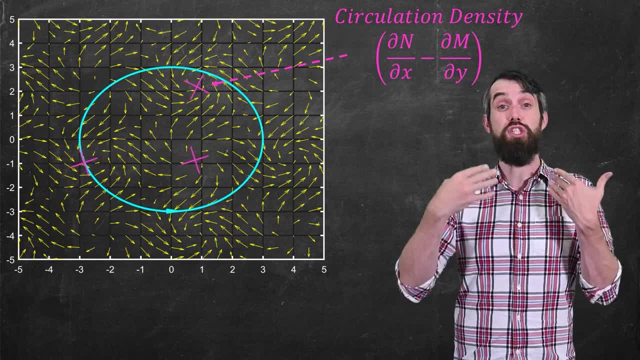 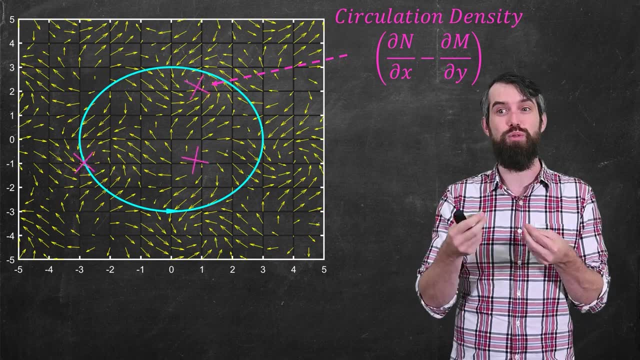 This notion of spinning at a specific point we'd previously called the circulation density and we'd seen how to come up with a formula for it, which was the partial of n with respect to x minus the partial of m with respect to y, and that measure gave a degree to which you'd have spinning at a particular point. 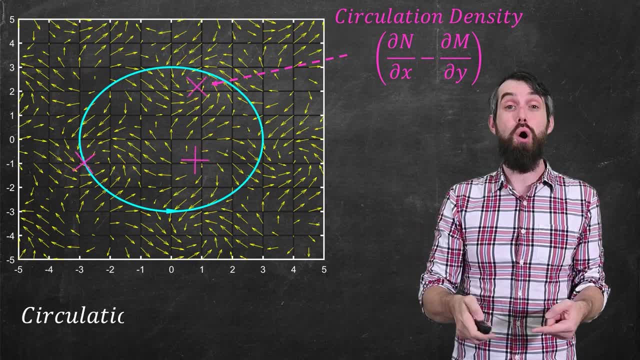 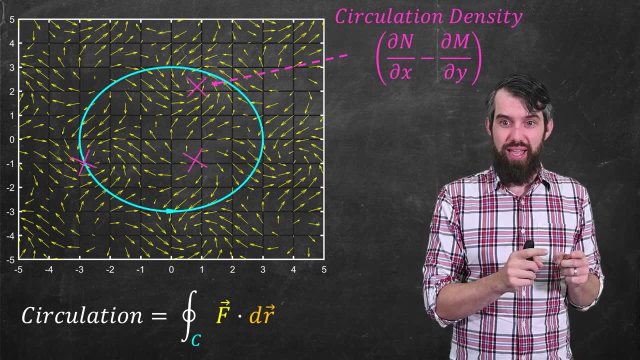 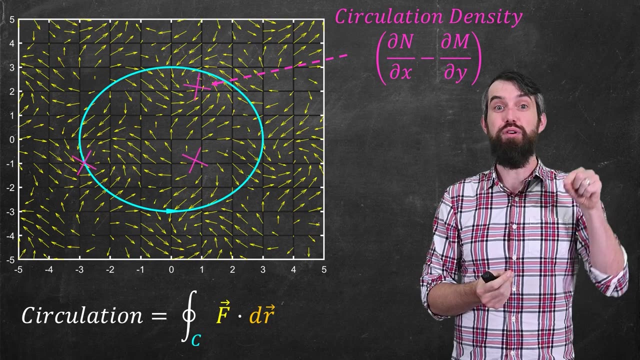 So that's a local property, but we've also seen what I'll call a global property, which is Now. the magic of Green's theorem is that these two different concepts- one a global property along a full curve, the other a local property at every specific point- can be related, can be stated in the same formula. 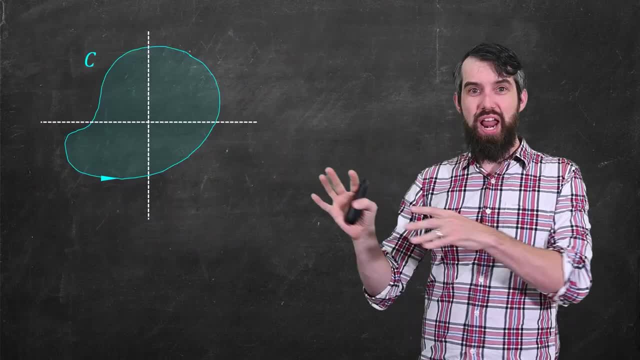 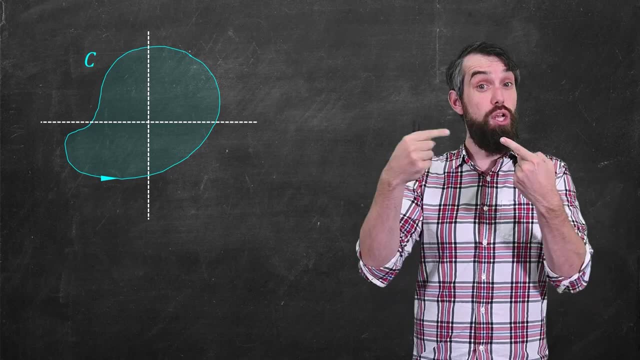 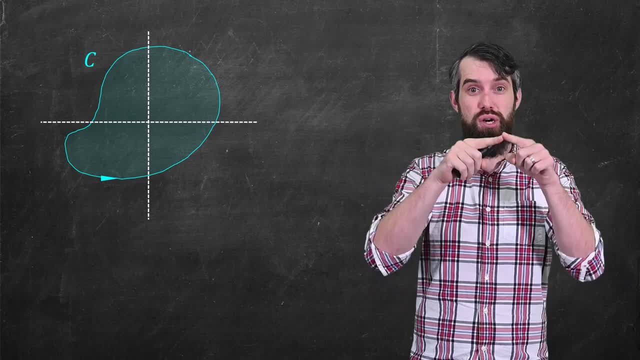 And later on we're going to have some conditions on this curve. For example, it needs to be a closed curve, That means it comes back together, And it also has to be what we call a simple curve, which means it has no self-intersections. 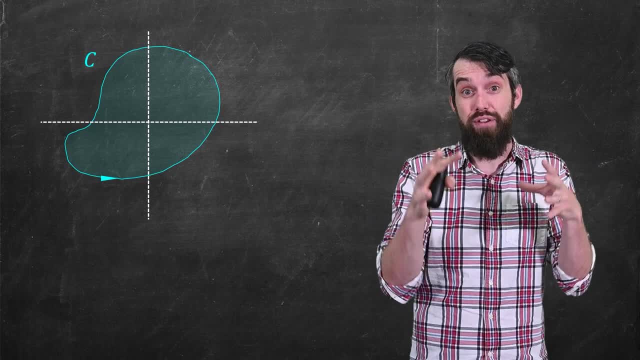 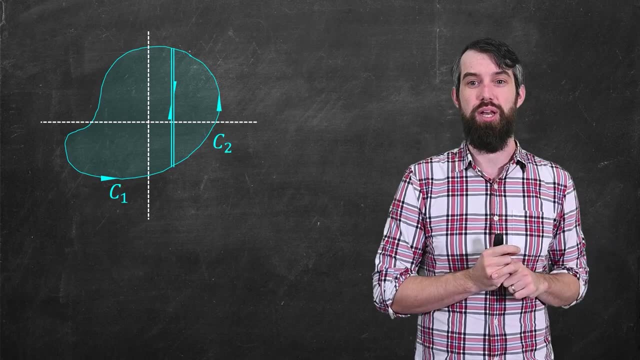 The point of these conditions are to talk about curves that enclose a specific region. Now, I could compute the circulation along this curve if I wished, But let me do something else. Let me cut this region. So I'm going to come here and I'm just going to cut it up and divide it now into two different regions. 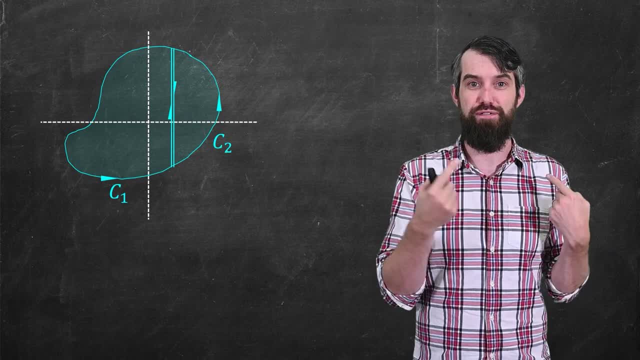 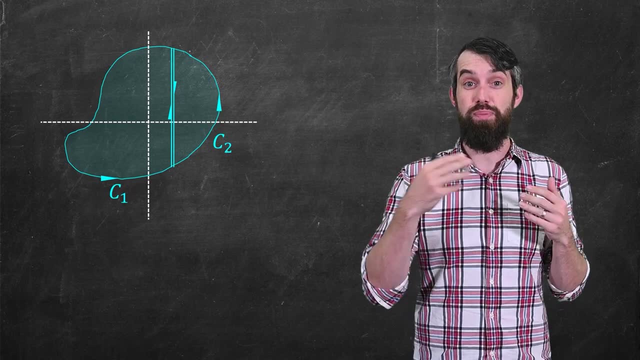 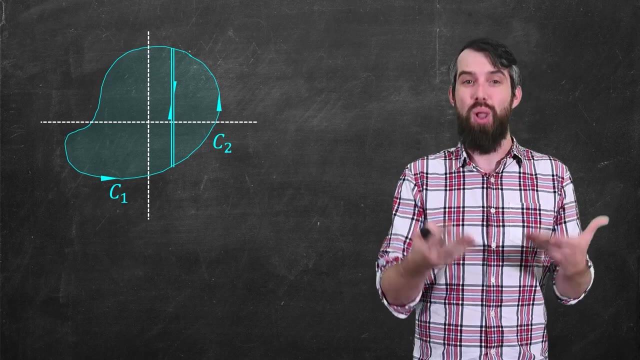 There's a C1 curve that wraps around The first region on the left and a C2 curve that wraps around the second region on the right. And then note carefully that to keep the complete counterclockwise rotation of the curve, that what happens when you go along the cut is on the C1, you're going up along the cut. 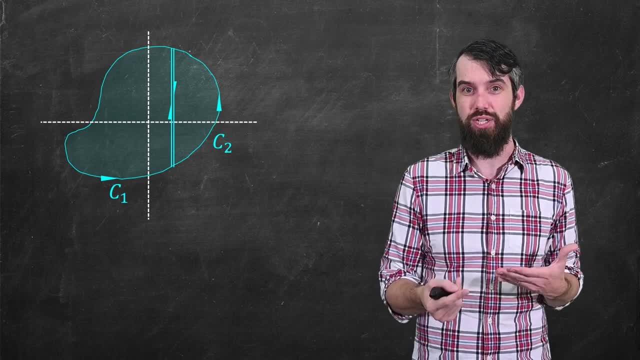 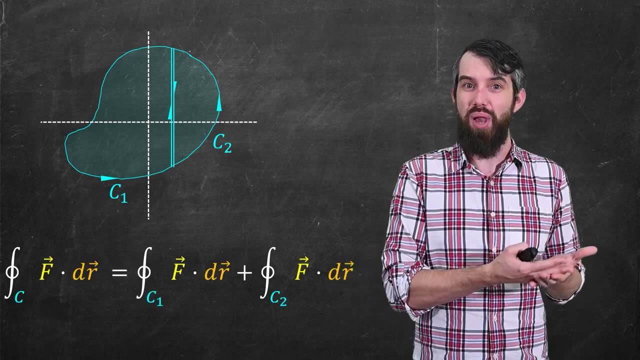 And along the C2, you're going down along the cut. They're in opposite directions. Now notice the next point, which is that if I compute the line integral along the broader curve, it's just the sum of the line integral along the C1 and the sum of the integral along the C2.. 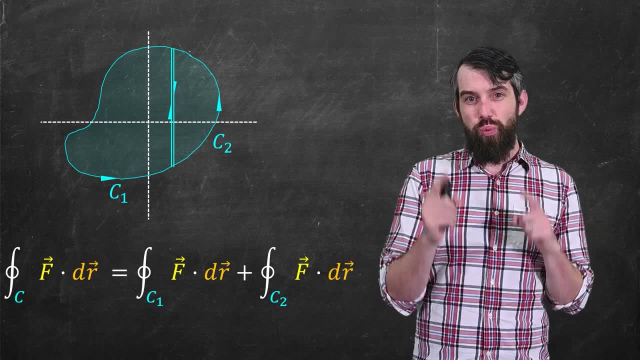 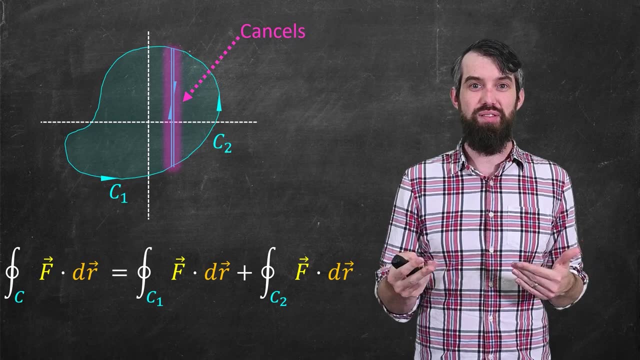 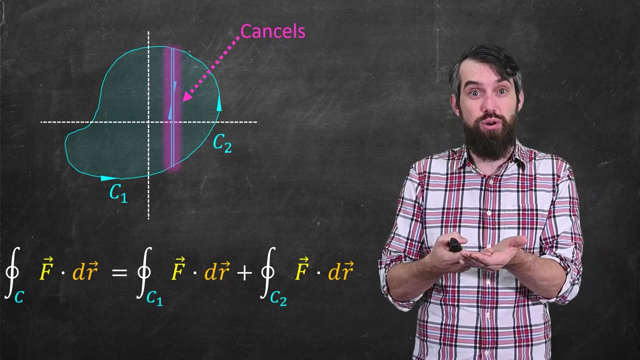 The line integral. It's just written as this: sum, And the reason this works is because along that middle portion here, well, everything just cancels The same line. it's just they're in opposite directions. So along one of the integrals, if it turned out to be, say, positive, along the other integral. 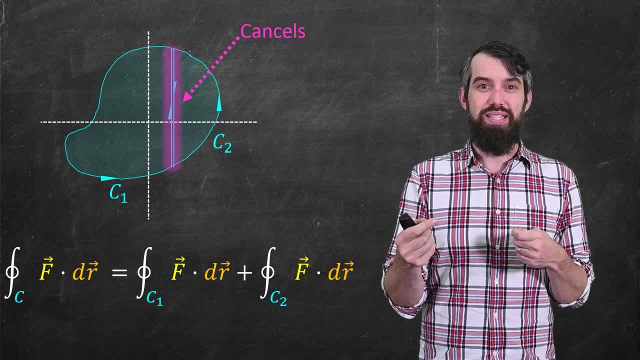 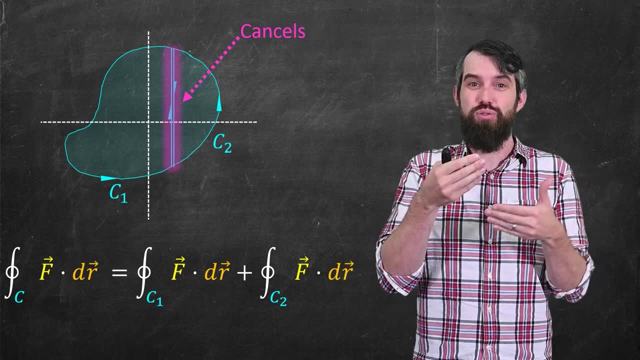 it would be negative because of the opposite direction. So the point is I can cut my region, create these two curves which, yes, they are longer in total length, but the extra length that's created along the cut, that just cancels out. 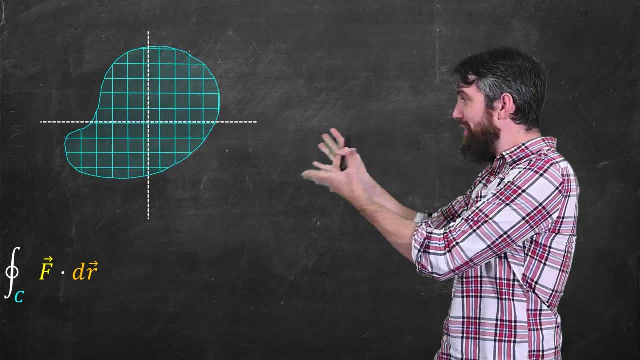 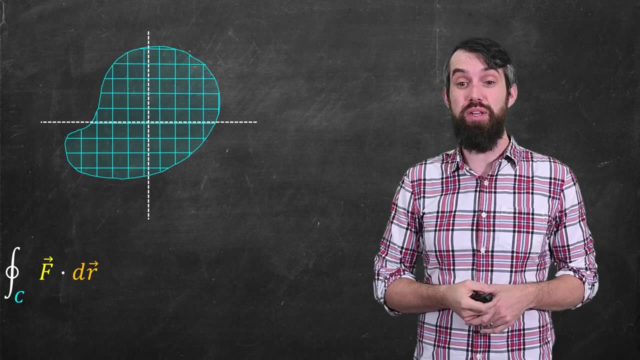 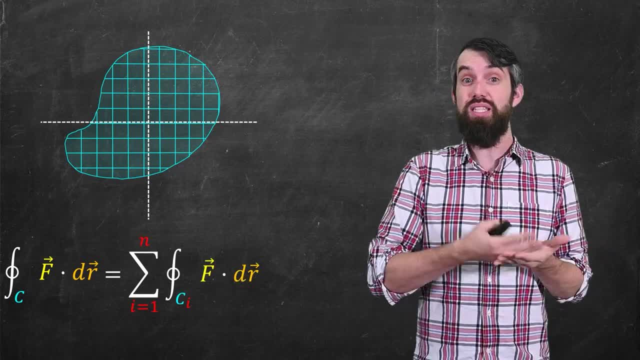 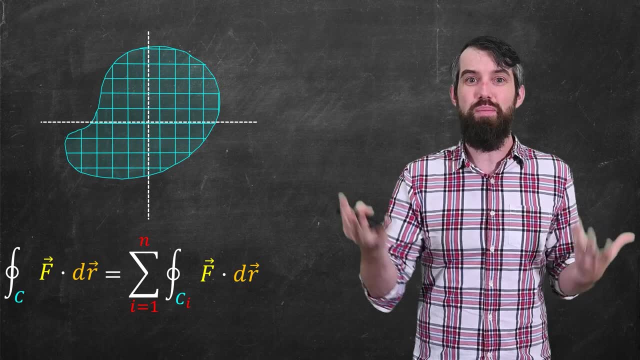 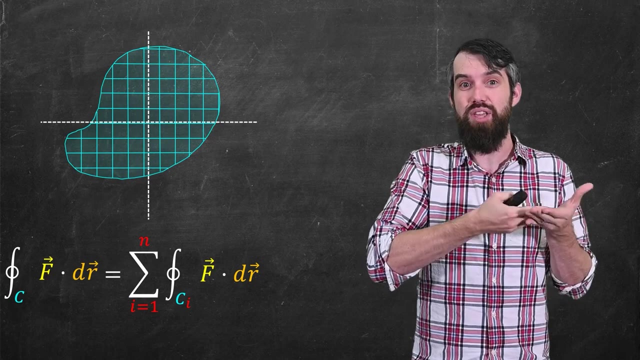 I could say my total line integral around just the outside was the sum of all the little line integrals around all the little regions that had been resulting from all of my cutting. Basically everywhere in the middle you just get internal cancellation. You have the line integral in one direction and then the corresponding line integral right back in the opposite direction. 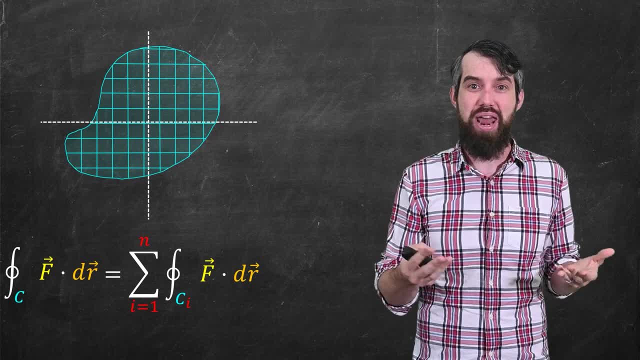 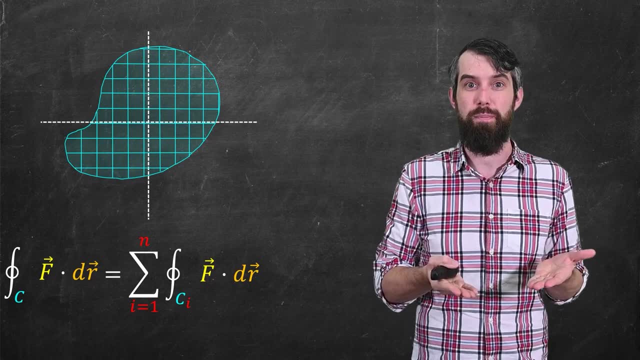 with a negative sign, And it's a negative sign being introduced. So all that's left when you add up line integrals around all these little rectangles, is nevertheless just the final boundary, the line integral just along the boundary. Okay, now here's where the real magic comes in. 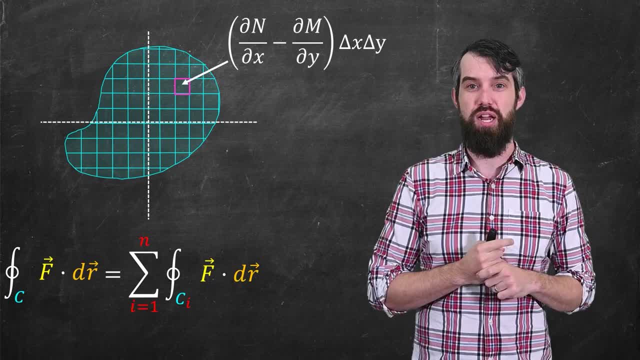 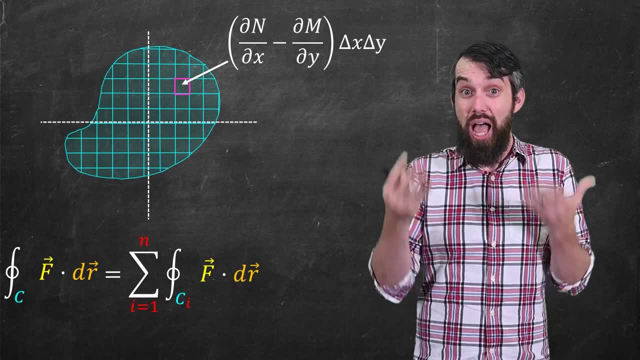 If I focus on just one specific little region here. so I imagine a tiny little rectangle and I'm computing. well, what is the circulation around that line integral? What is the line integral going to be? Well, in our previous video, when we introduced the notion of circulation density, 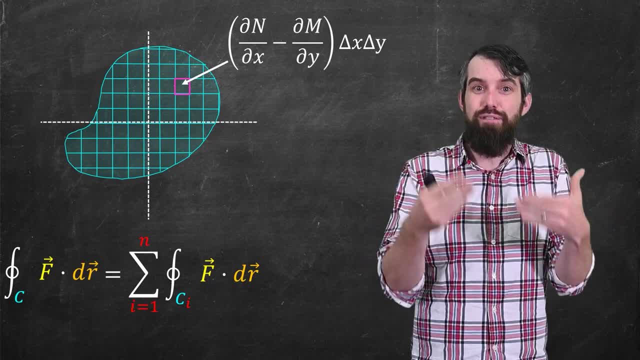 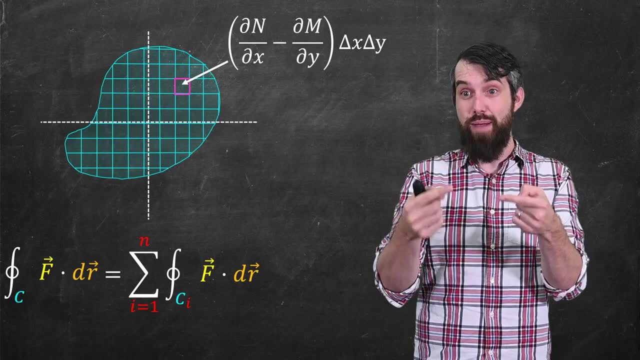 we computed that the line integral around that line integral is going to be the same as the line integral around the other line integral. line integral around some infinitesimal rectangle could just be given by the circulation density partial of n with respect to x minus the partial of n with respect to y. 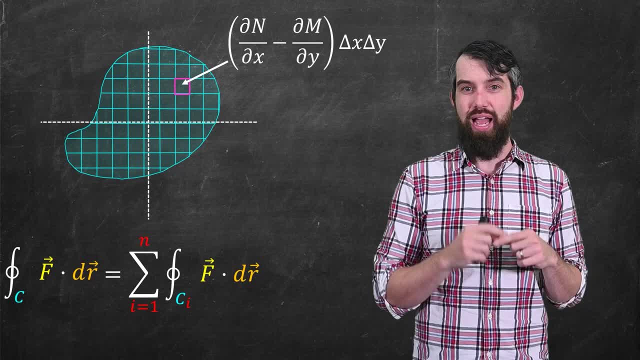 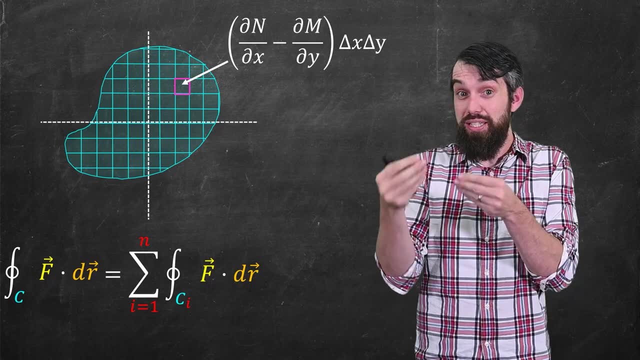 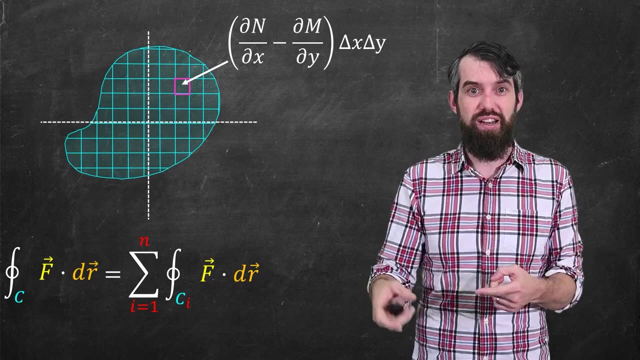 times the area delta x, delta y. And so now I'm starting to get this relationship between the total circulation around the entire curve and then the circulation density around these tiny sort of infinitesimal rectangles when I cut it up more and more and more. So if I take the limit as n goes to infinity. 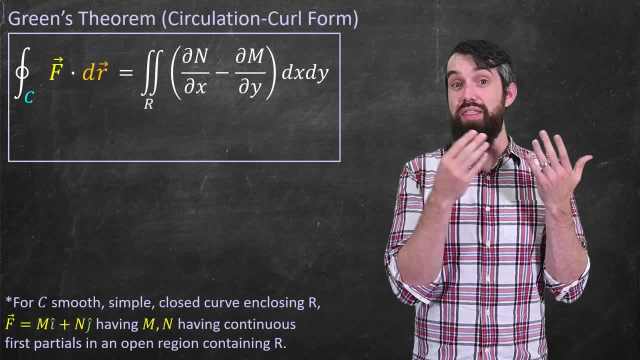 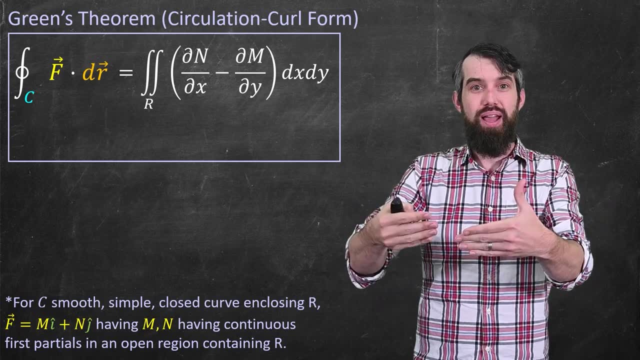 what I get is called Green's theorem And it says that the line integral around a curve is: you just take that circulation density and you add it up, add it up, add it up and a whole bunch of accumulations. this is just a double integral. 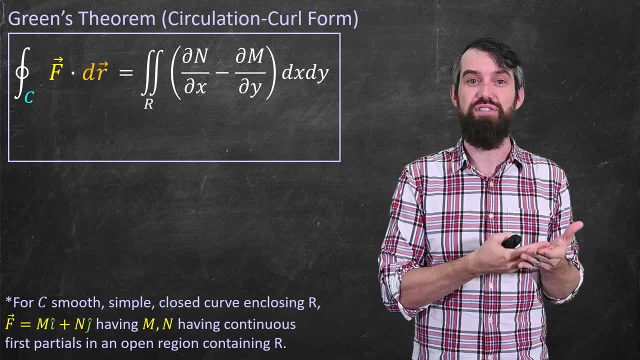 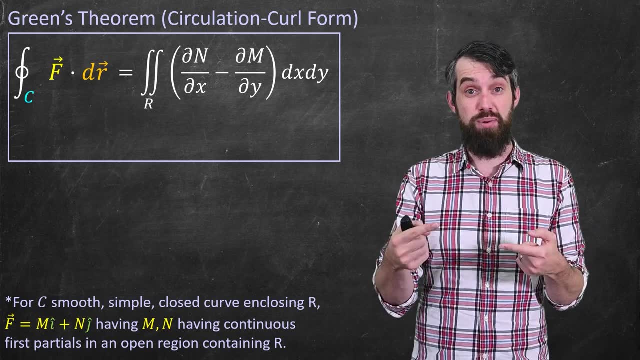 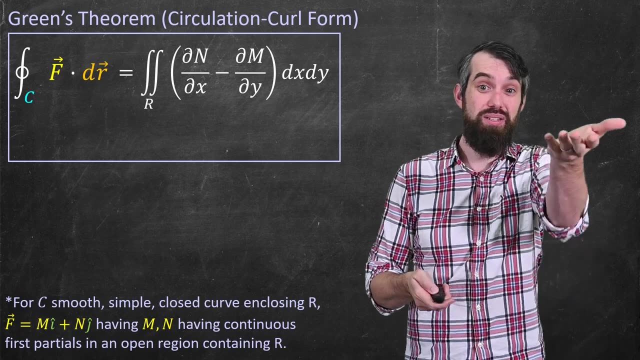 So, in other words, the line integral around the curve, the f dot, dr, is the double integral over the enclosed region of the circulation density and then integrated with respect to the little area, this da or dx, dy if you prefer. So basically, what I'm saying here is that on the left, 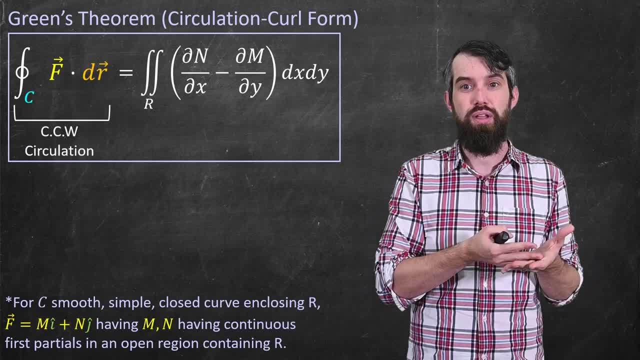 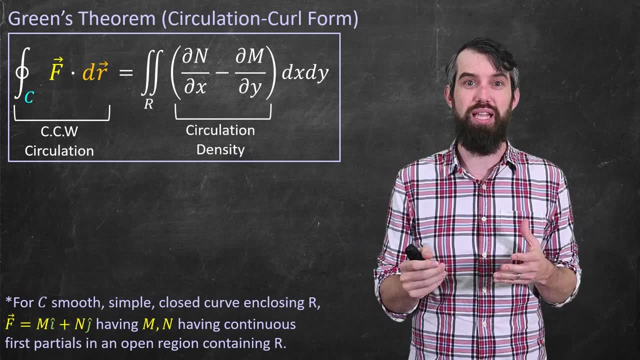 I have my counterclockwise circulation as I go around this curve And then on the right-hand side I am integrating the circulation density. So Green's theorem in its circulation curl form is just saying the total circulation is just integrating up over all of the area. 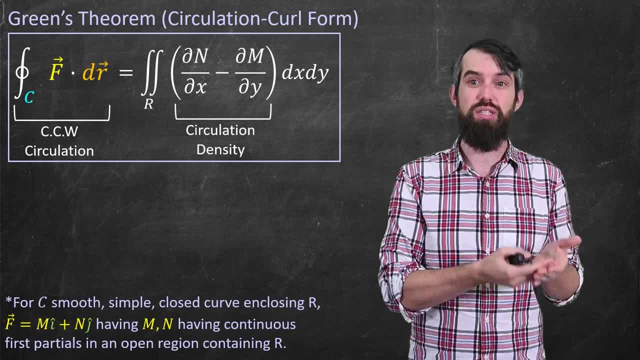 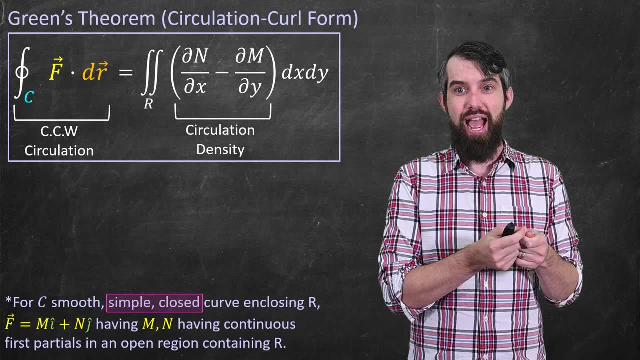 of the circulation density. I have some regularity conditions on my curve and on my field. They have to be relatively nice. The most important of those conditions is specifically that it's a simple closed curve And that was going to imply that we had a single region r. 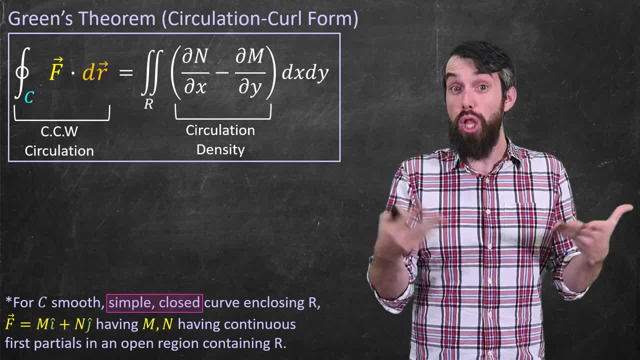 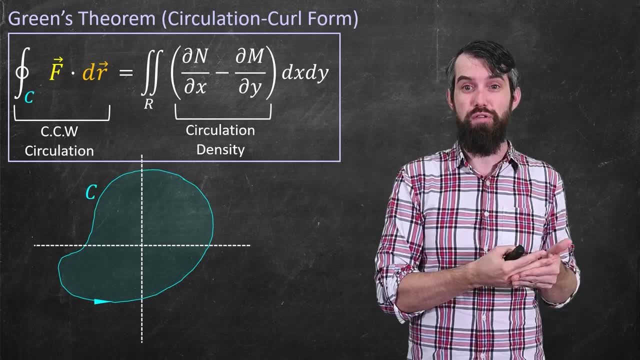 that could be described from our particular curve and the region was enclosed by that curve. Okay, so to help visualize this again, if I have my region enclosed by my curve and I'm trying to take the circulation around the boundary of that region, then I can imagine at any point here: 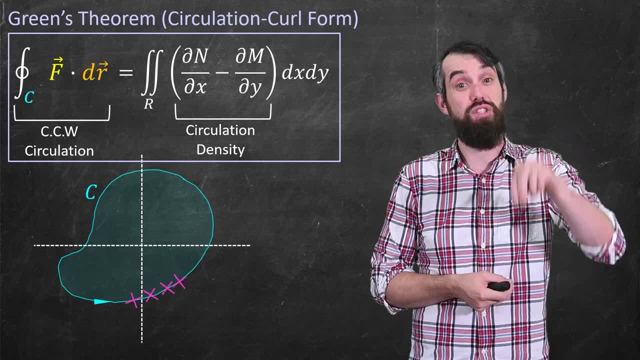 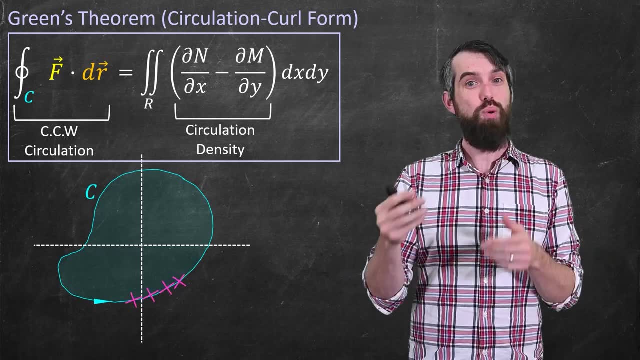 I can have a whole bunch of different little spinners where I come down and measure the circulation density. I just put four, but it would go all the way around the boundary and indeed all the way in the middle And then at each point along the boundary. 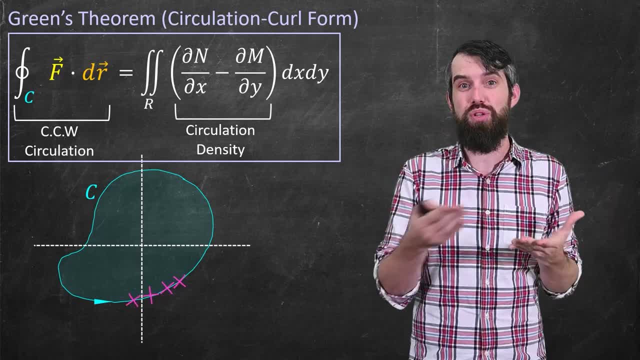 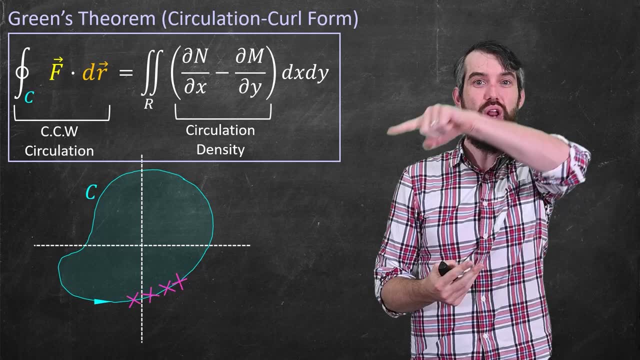 this tendency to spin at that particular point is going to contribute to that portion of the circulation along the boundary. Now, this would seem very strange, because circulation is something that only occurs around the boundary. It doesn't matter what's going on on the inside right.